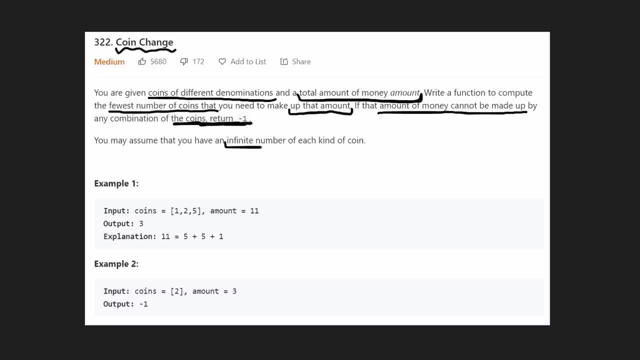 the case And luckily for us, we're actually given an infinite number of each coin. So in the first example we have coins of value one, two and five and we have infinite quantities of these coins. The amount that we want to sum up to is 11 and basically you know, just look at. 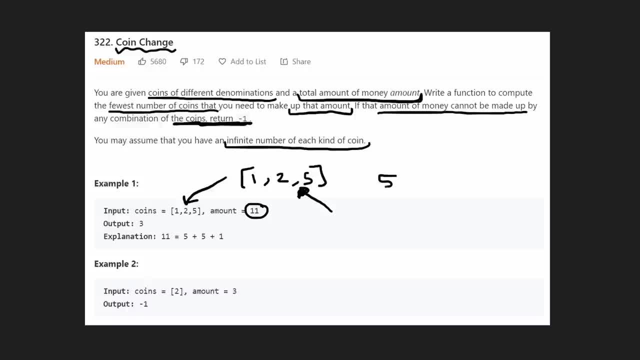 this: What's the fewest number of coins we could do? Well, of course we want to use a five, because it's the biggest one. We can use another five and then we just need a one left if we want to sum up to 11.. So in this case, you can see, we only needed three coins. This is the fewest number of coins. 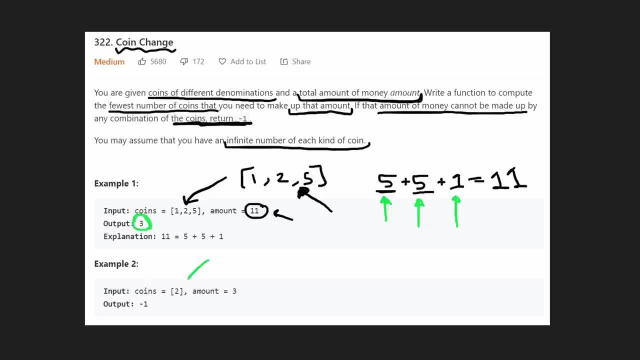 we needed, so we can return three. In the second example we have a coin of value two but we want to sum up to three. We can try two plus two, but we know that's four, so we went over three. So there's no way to possibly sum up to three, so we return negative one. There's no possible solution. 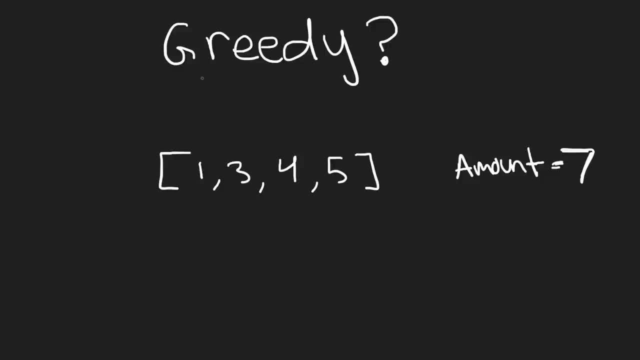 So your first idea might be: can we just be greedy? Is the problem that easy? Can we just be greedy? And let's look at this example. So let's say these are our coins: one, three, four, five, and we want to sum up to seven. So when I say greedy, I mean okay, we want to sum up to seven. Let's just start. 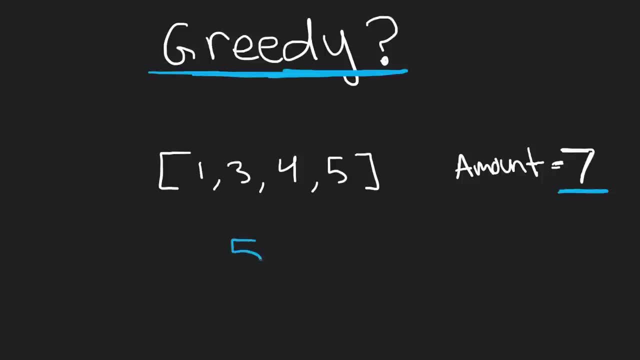 at the biggest coin we have. So let's start at five. So now let's look at the biggest coin again: five. If we add a five here, we know we're going over. we're going over the total amount seven, right? so we don't add another five. Well, let's look at the 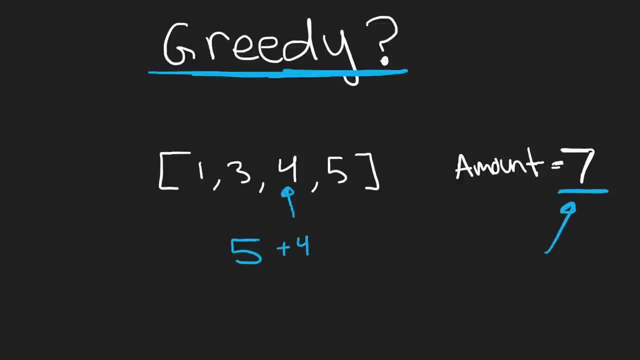 four. Well, we know, five plus four is also going to be more than seven. Five plus three is going to be more than seven. Okay, but we found a one. Luckily we have a one, so let's add one to it Now. we're at six, So let's add a second one. Now we got to the sum seven. 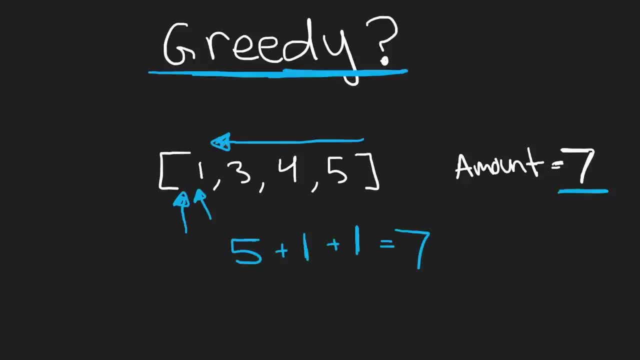 went down from the biggest smallest coin values. right, that's what i mean when i say greedy, let's pick the biggest one possible first. so notice that this took us three coin values, right? so our result in this case would be three, but is that the minimum amount of coins? the answer is no, because 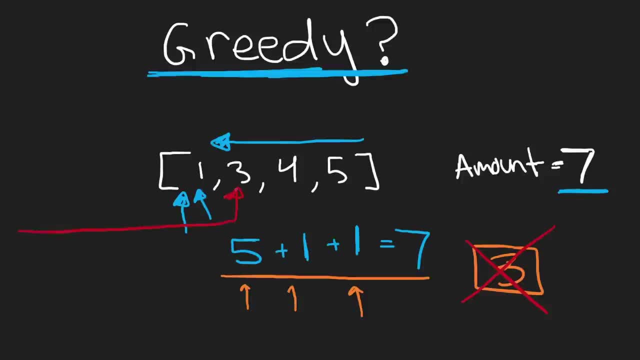 you know, just looking at it we can tell we got a three and we have a four. three plus four is seven. that means the minimum amount of coins is actually two. so this is a counter example. we cannot be greedy if we want to solve it. so the next thing you might try is like a brute force solution, right? 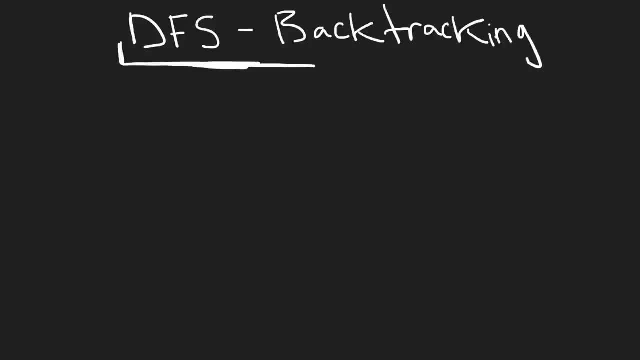 so to do the brute force solution we need to implement some kind of depth first search or backtracking solution. right, so you know, just looking at it we can tell we got a three and we have a four. three plus four is seven. let's look at the same example: one, three, four, five and amount sum to seven. so what would a? 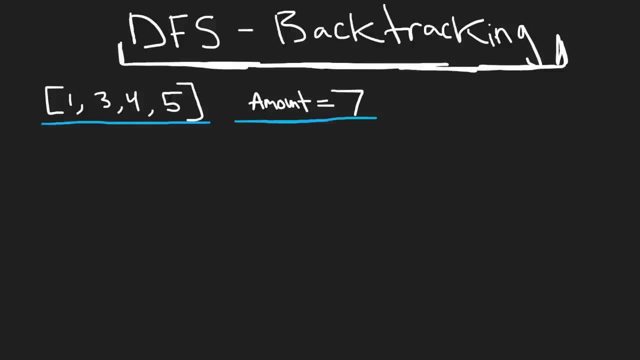 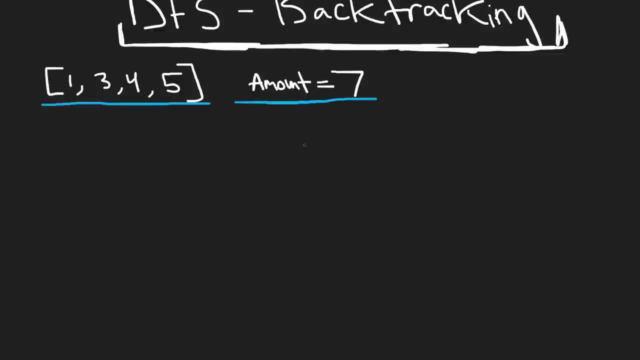 backtracking solution even look like for this problem. well, it's going to be brute force, right? so? so we have four coin values. so that means in our decision tree we have four possible choices. we can choose a one, we can choose a three, we can choose a four or we can choose a five, in this case. 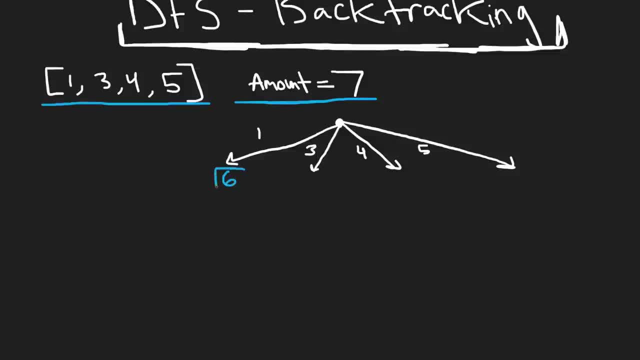 the remaining amount would be six, because we have a three and we have a four, and we have a four because seven minus one is six. in this case, the remaining amount that we have to compute would be four, because we're taking seven minus three, which is the coin that we chose, so we get. 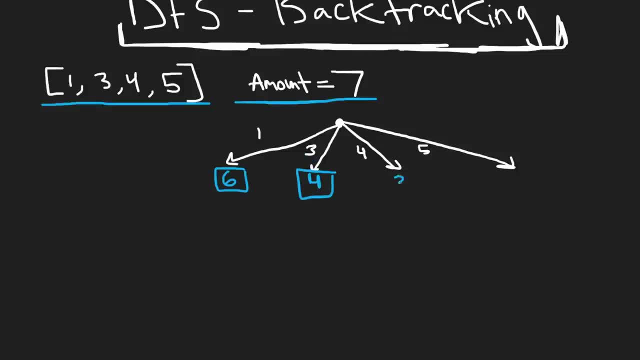 four as the remaining amount, right, in this case we would have a three and in this case, we would have a remaining amount of two. so, since none of these are zero, once we get to zero we know that that we've computed the total amount that we want to compute and we're going to have a three and 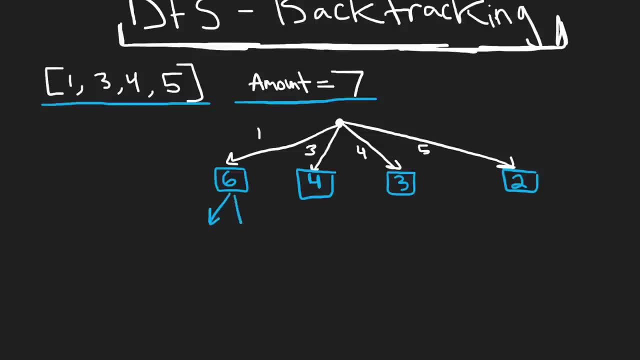 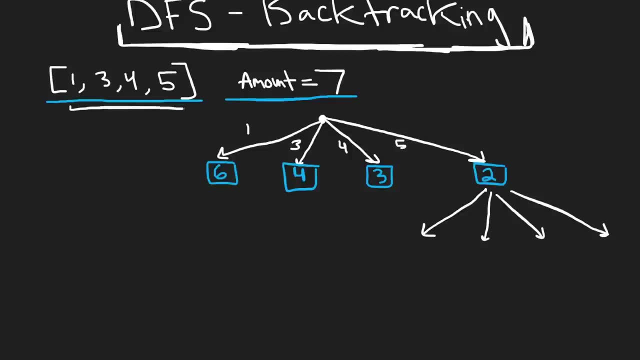 single question. right now, we're going to have a liquid five and we're going to have a nine into four. we can either, because of the risk, as happen in this case- we couldn't really compute anything, save the amount of time- and we can, um, we can take the negative1 which we already set in the 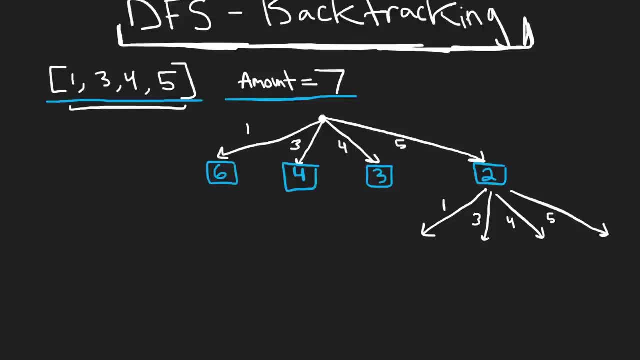 scale function. so the negative 1 will help us calculate what our rupee balance would cost, which is the samearts required, for which one will be money. so we just have to calculate the amount of time. and second and third, because we've been COM, still known for what we've been- 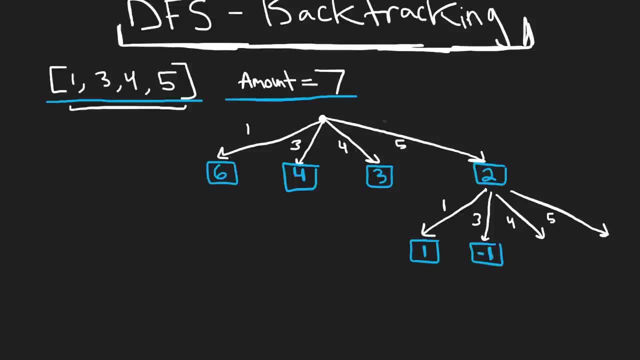 calculating. so that's exactly what it was, because we came up with the negative one. what happened here? okay, let's see where we're going to have the negative one. we don't have that much, do we actually five coin and we chose a three coin. then we get to a negative value. that means five plus three. 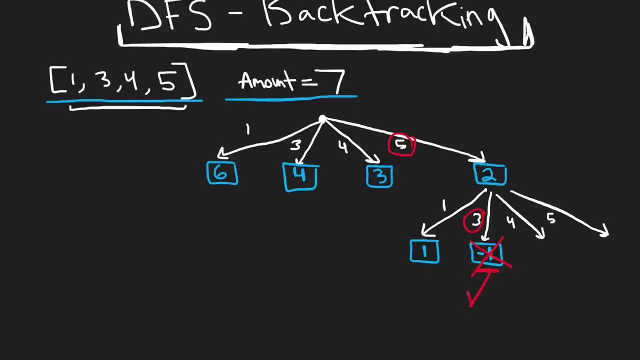 cannot be the amount, so we don't have to keep searching here. we can stop right. we got to a negative value. if we keep adding values to it, it's just going to become more and more negative, right, and you can probably notice that since these values are even greater. two minus four is going. 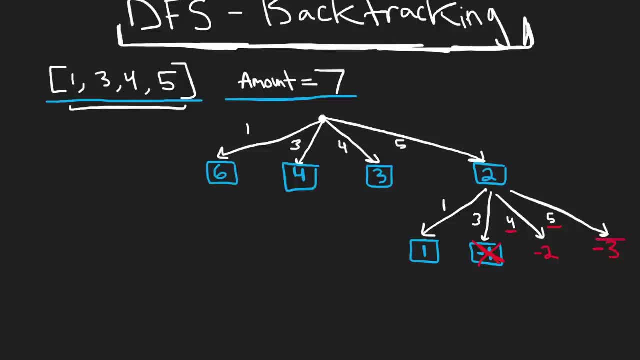 to be negative two. two minus five is going to be negative three. so we can't go down these paths either. we don't have to search them anymore. and so now, here we're going to see: okay, we can choose a one coin. of course we can choose a three, four and five, but we can see from here that that's not. 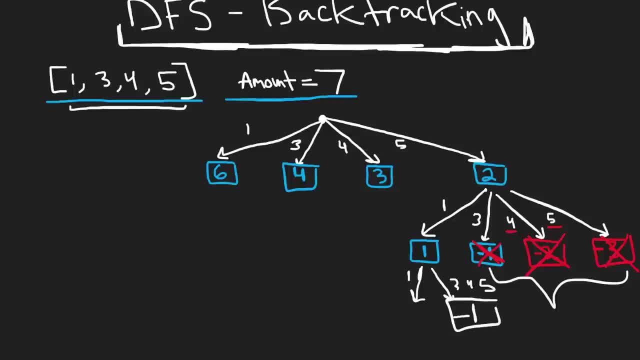 going to work. that's going to lead us to a negative value anyway. if we choose a one over here, then we know we're going to finally get to a zero. so this is what we want, right? we took a five from up here, we took a one from over here and we took 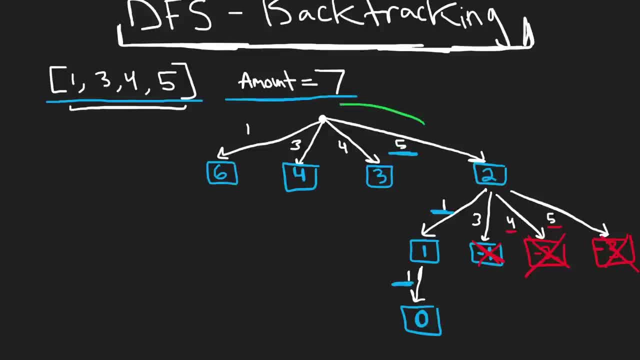 a third one right. so then if we count how many coins we chose down this path, we know we get three coins right and we get to a zero. so of course we don't have to keep searching anymore. so we found one possible way where we can sum up to the amount seven. we know it has three coins which 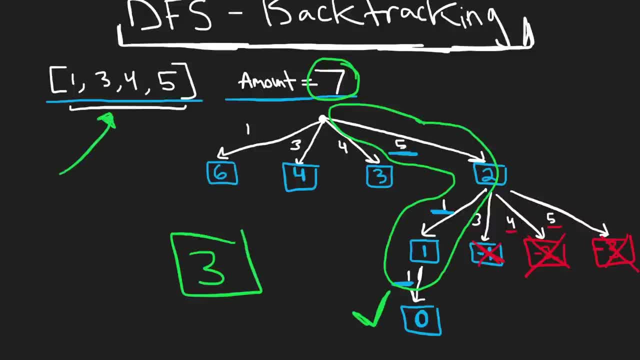 you know from the previous example, we know that that's not the minimum amount of coins, but we found an algorithm that at least tells us a possible solution so we can kind of keep track of that, the minimum coins we can set to three. so now i'm going to show you what happens when we go down. 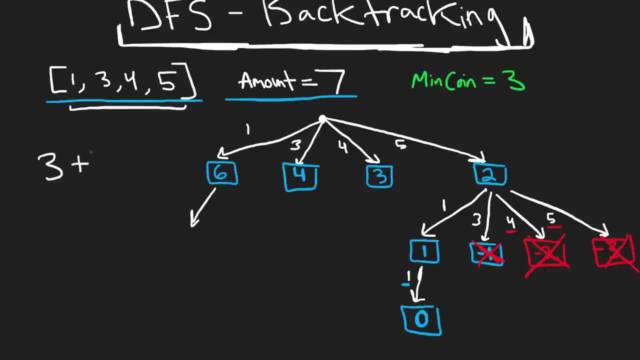 this tree path, even though we know that the solution is actually three plus four, which is two coins, which either of these is gonna get us to the correct solution. i'm going to show you what happens when we go down this tree path and we know that the solution is actually three plus four. 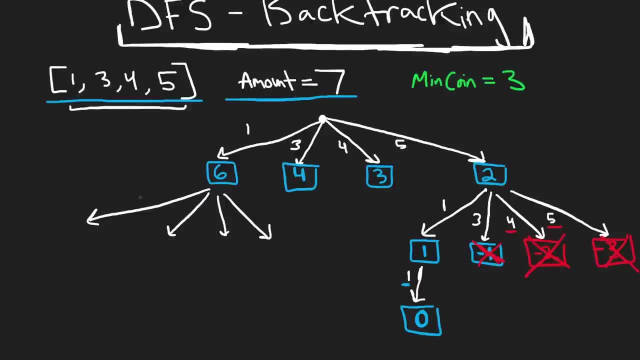 and we go down this one anyway. so we can choose a coin: one, three, four or five. so if we go down this path, we will have a remaining amount of five. here. we'll have a remaining amount of three. here we'll have a remaining amount of two. here we'll have a remaining amount of one. do you kind? 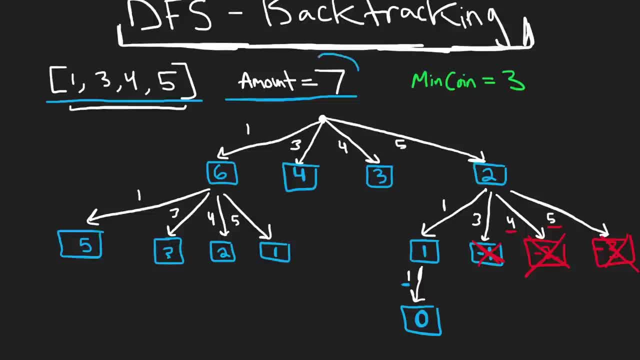 of see how we're taking the original problem, which is seven, and then breaking it down into sub-problems like six, and then breaking it down even further into five. And not only that. we have subproblems, yes, but do you also see that these subproblems are repeating themselves? Here we have a remaining. 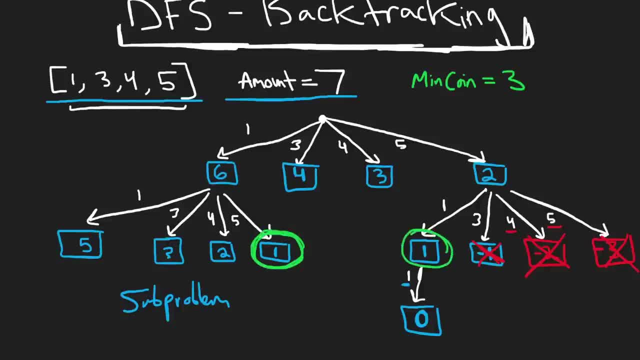 amount of one. Here we also have a remaining amount of one, So do we even have to compute this path, Because we already know, if we have an amount one, it takes only a single coin for us to be able to reduce it to the amount zero, which is what we're looking for. So, since this subproblem 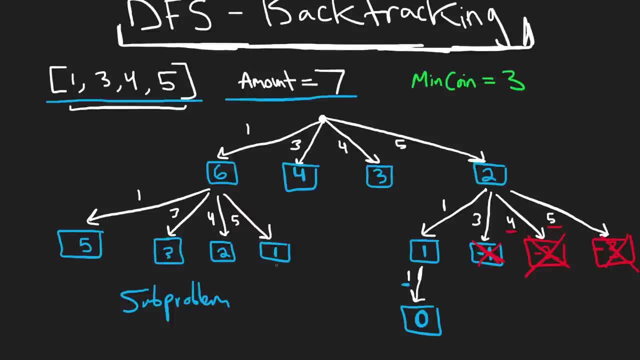 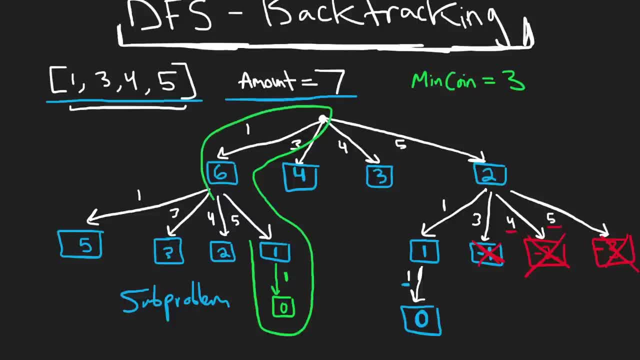 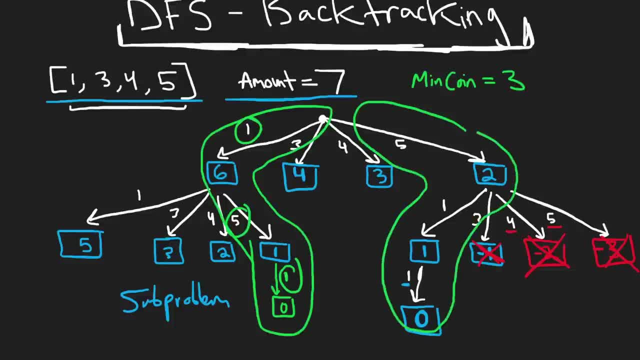 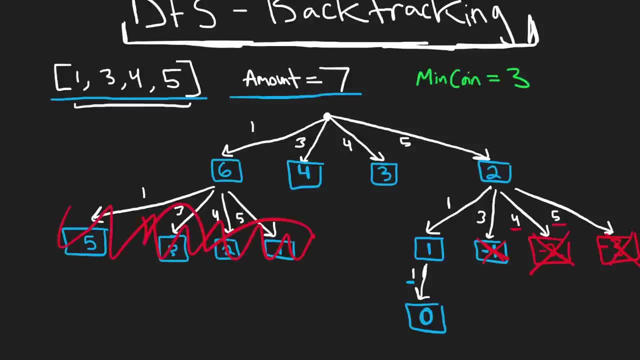 basically, we got the same thing that happened over here, just in a different order And just to make this a little less messy. I'm just going to tell you that none of these are going to lead us to the optimal solution. So now let's look at this case. We have a remaining amount of four. 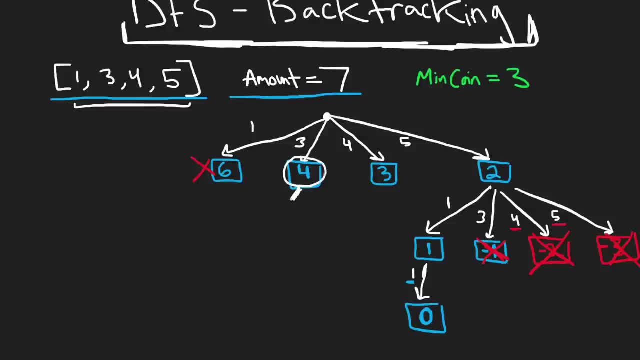 How many coins does it take for us to get an amount? four? Well, let's brute force it. Let's check every possible combination. Here we'll get a one. Here we'll get the value we're looking for: zero. That's great, But let's just look at this last one. 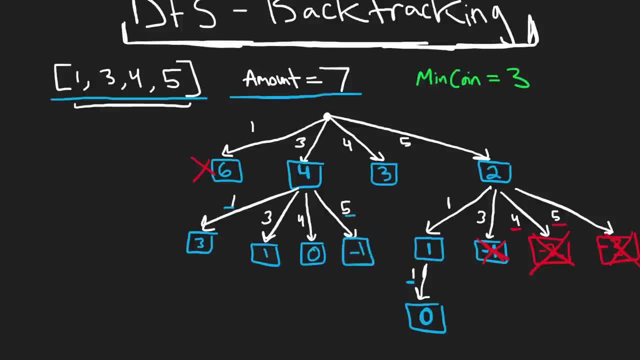 with five, We'll get a negative one, meaning we can stop searching. So this is awesome. We got a zero, And let's count how many coins to take us to get to this zero. We took one, four and we took a three, So this path is only two coins long. We. 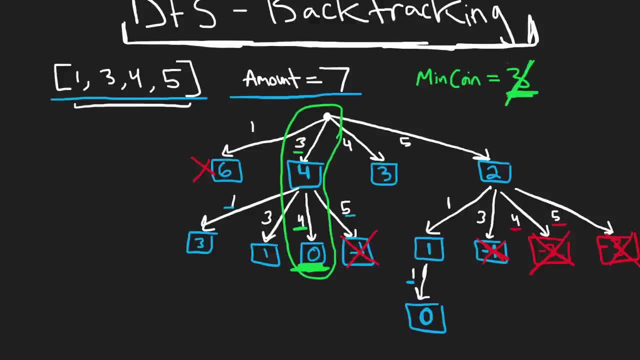 see, our minimum is currently three, but we can actually replace this now with a two, because two is the minimum number of coins needed to total to amount seven. So we know this is the correct answer, but let's just see what happens with the remaining stuff. So first let me just look at this. 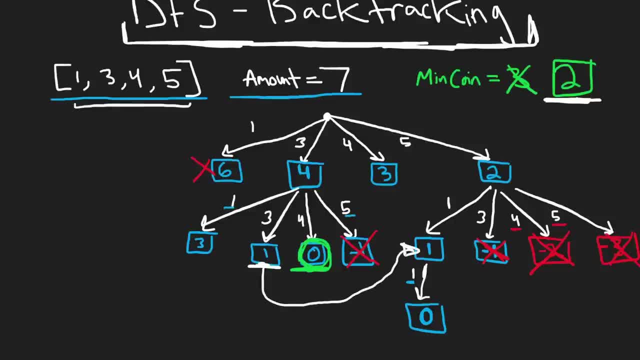 one. We see we actually already solved this sub problem over here, so we don't really need to solve it again. We know it takes one coin for us to go from one to zero. And what about this three? Okay, well, we can do the same thing, right? One, three, four, five. 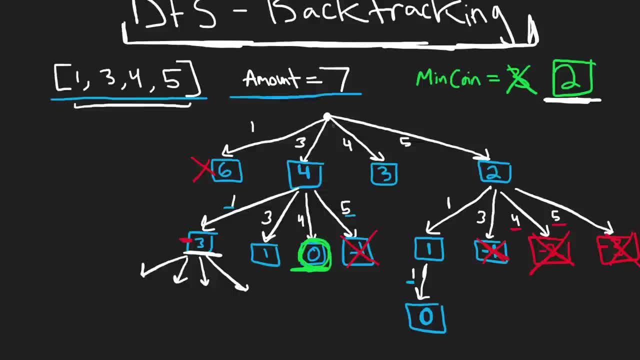 And I'll just tell you from here, we're not going to find the optimal solution. going from four to three and more, That's going to obviously be more than the current minimum of coins that we have, which is two right now. So this is not going to lead us to the correct solution. But you see, 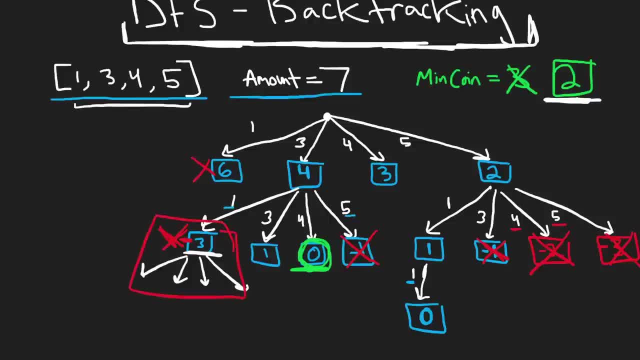 that once we compute this stuff then we have one Last subtree over here, right, This original three. But once we already solved the sub problems of this, do we really have to solve the sub problems here? No, If we store it in memory, if we have like, 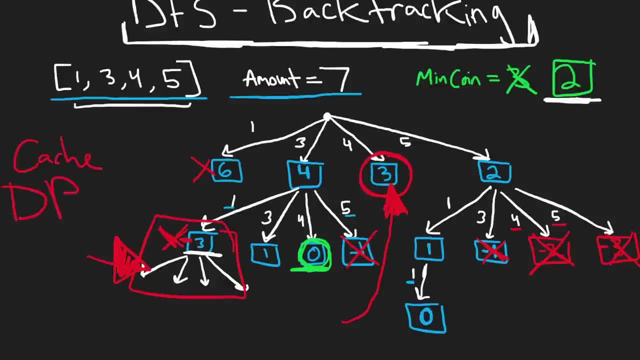 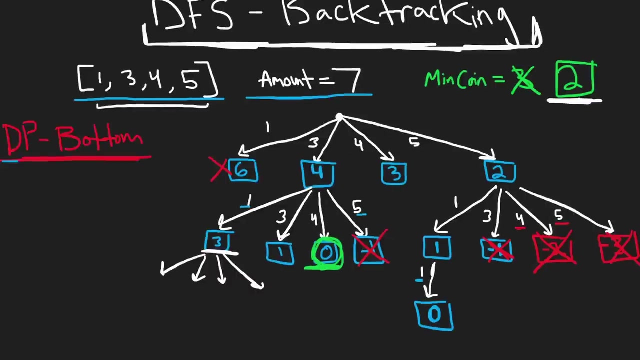 a cache, or you can call it DP. we do not have to repeat these sub problems. So the way I just solved this was called top down or top down memoization, So bottom up, basically, instead of solving the original problem where the amount is seven. 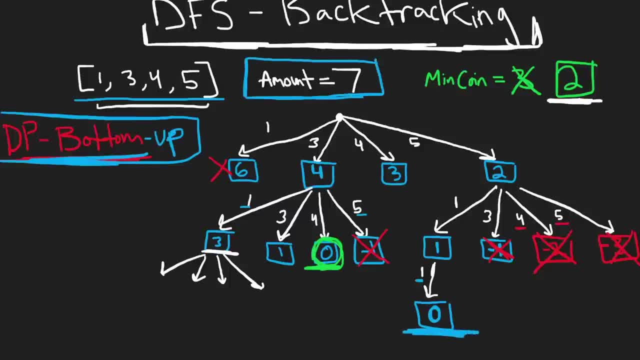 we solve it in reverse order. We start at the smallest one, which is zero. right, This zero over here. So we want to know what's the minimum number of coins. We can call it DP, DP of zero. So for amount equals zero, what's the minimum number of coins for us to sum to zero? 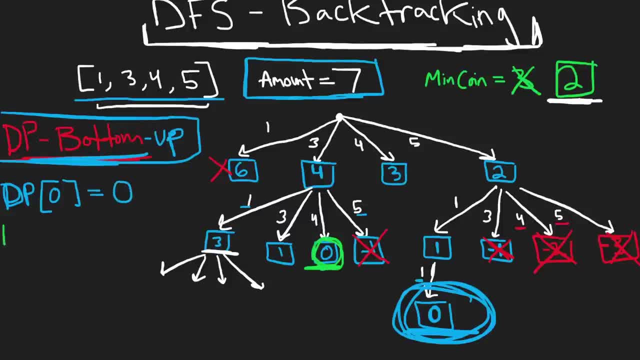 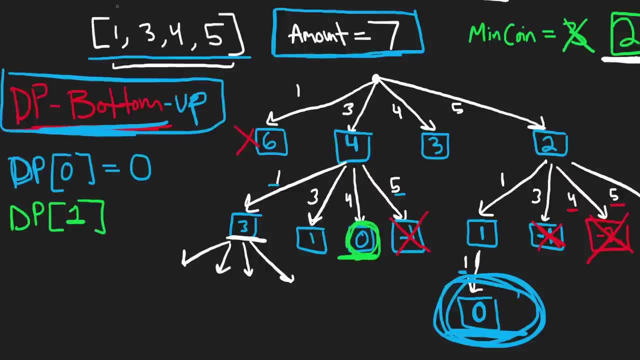 Well, we know it just takes zero coins, right? What about if we want to know what's the minimum number of coins for summing to one? Well, we can look at our coins. We got a one, a three, a four and a five. These will all cause it to be greater than one, but we just want a one. 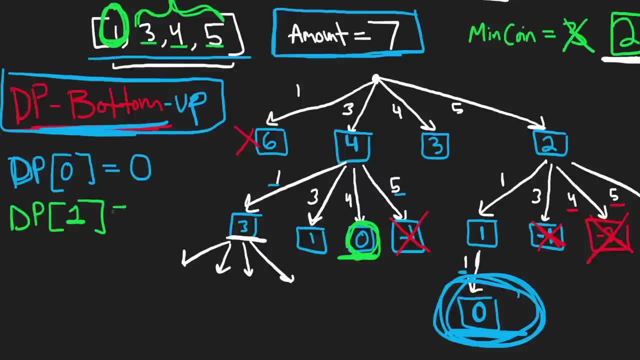 So we can take just this Meaning: it only takes us one coin to sum to one, And then we can just repeat that process, right? So for a DP of two. so we want. how many coins does it take for us to sum to two? Well, we got four. 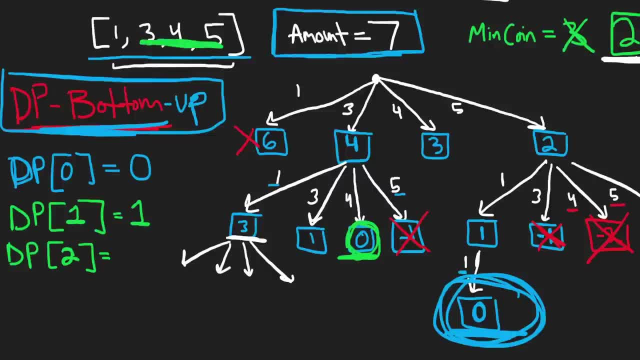 coins. right, These three will cause it to be greater than two, So we don't use those. But what about this one? Okay, we get a one, So it takes one coin to sum to one. but that's something we already knew. So if we want to, 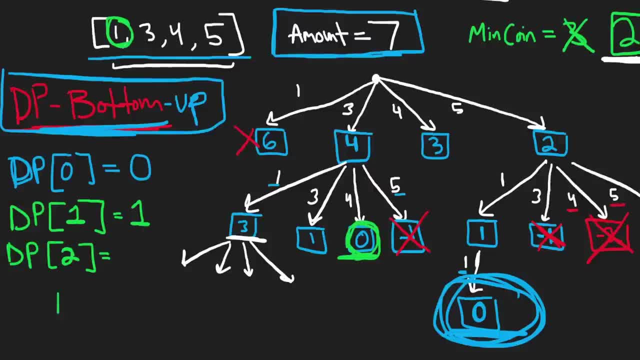 compute DP of two. we can take one plus DP of one, Because we know these three coins are going to be too big, but we have a one over here That's value one, And we also know that that's not enough, right? Two minus one still leaves us with a remaining amount of one, But we just 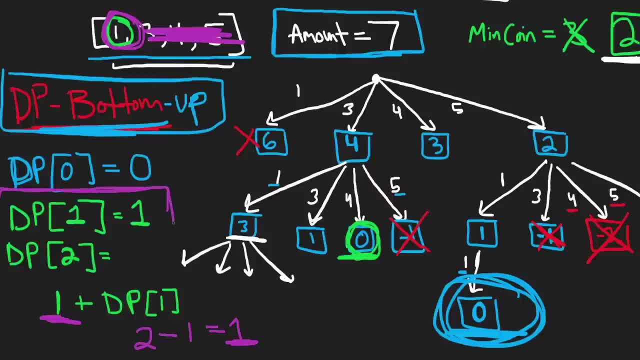 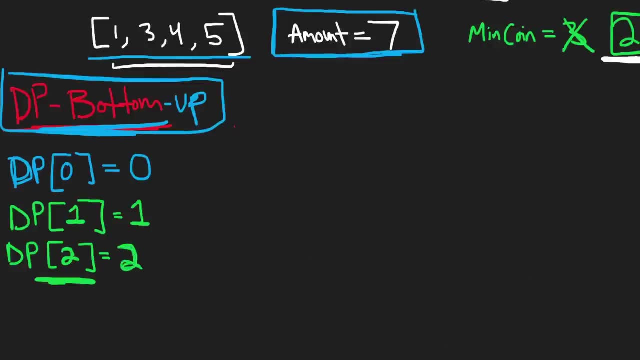 computed that up here. We know for us to get the minimum number of coins to get a value one, it only takes one coin. So that means that if we want to get amount two it takes at least two coins. And let's say we repeat this process. 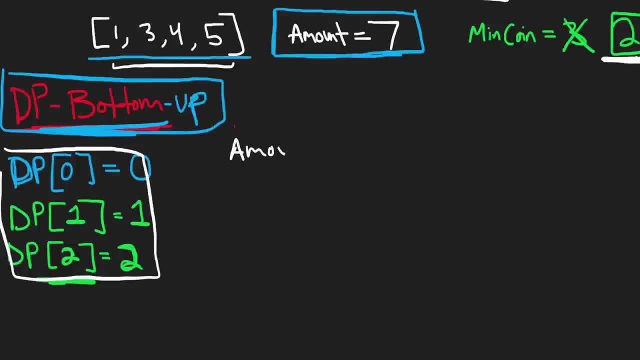 for all values, for all amounts, from all the way, starting at zero, all the way to seven over here. So I computed it from all the way, from zero to six, but the last time I did it it was seven. So the last one we really, really want is: amount equals seven. So let's compute. 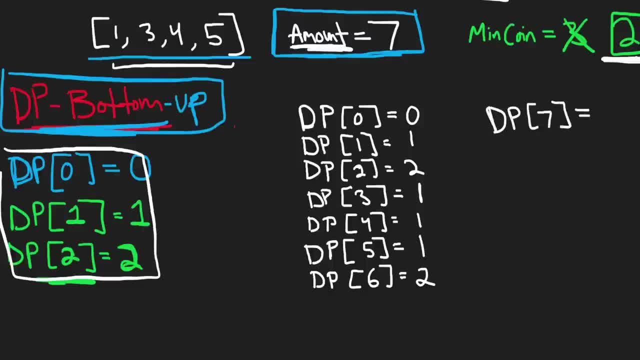 that DP of seven. How do we get it? Well, we still kind of have to check every single coin. So what happens? if we get coin one, then we are. then we take the result of one, meaning that's how many coins we use, not the value one, because we needed one coin. 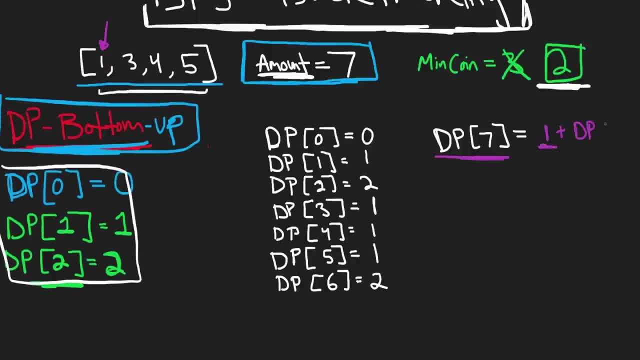 with a value one, And now we have a remaining amount of six right DP of six. So how many coins did it take for us to compute DP of six? Well, we already computed that it took two. So we get one plus two equals three. So that's one possible solution, but is 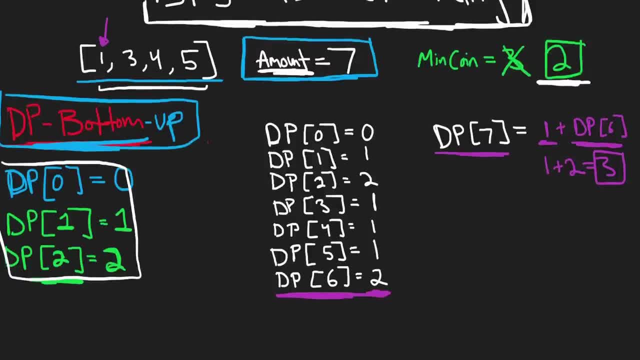 it the minimal solution. Well, let's look at if we use the coin value three over here. Well, it takes us one coin, So we take one plus DP of four, because that's the remaining amount we have to use. if we take a coin value of 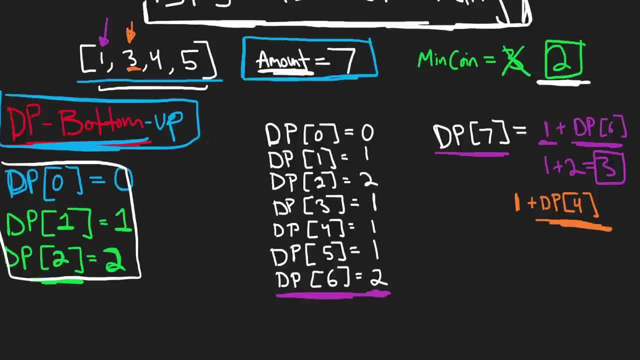 three And lucky. luckily we already computed DP of four. It is one. So then we get one plus one equals two, And we know that this is the real result that we want, But even before we know that we would repeat this process. So technically, if we do the bottom up dynamic, 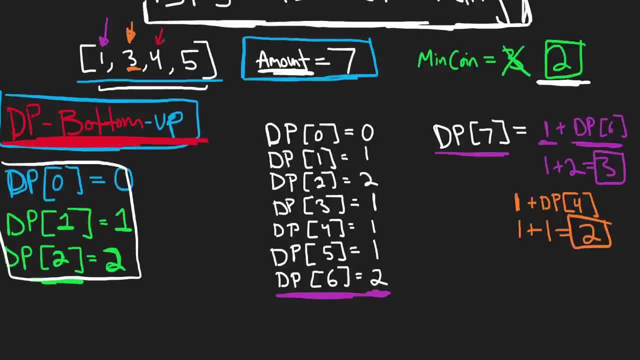 programming solution. we are going to repeat this process. So technically, if we do the bottom up dynamic programming solution, we are going to repeat this for the remaining two coins. So for four we would get one. So we'd have one plus DP of three. 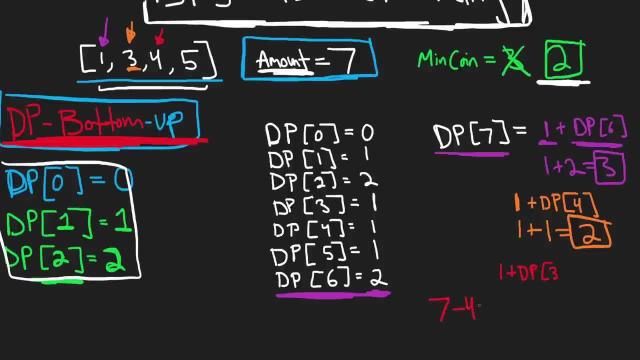 because four mine or because seven minus four would leave us with a remaining amount of three, And in that case we know DP of three is one, So we would have the total of two again. So we see that there are actually two solutions And we know we have one last coin that we technically 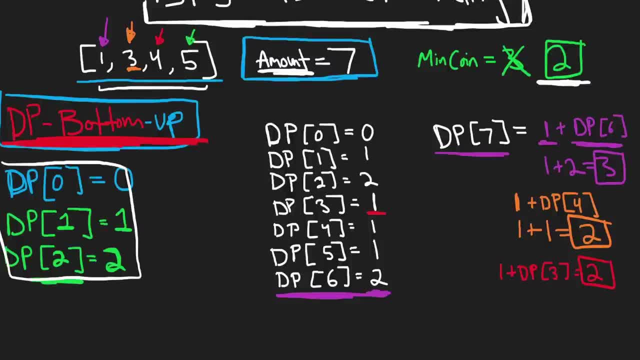 have to check Coin five. So we'd use one plus one equals one, So we'd have one plus one equals one coin for value five. And then the remaining amount we'd want to compute is DP of two, And we know that DP of two is value two. So this would result in a three, which is not what we want. 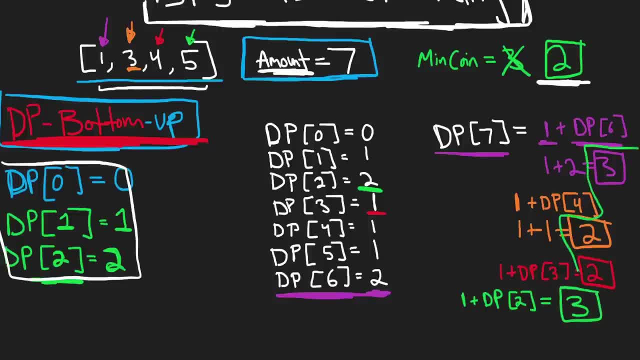 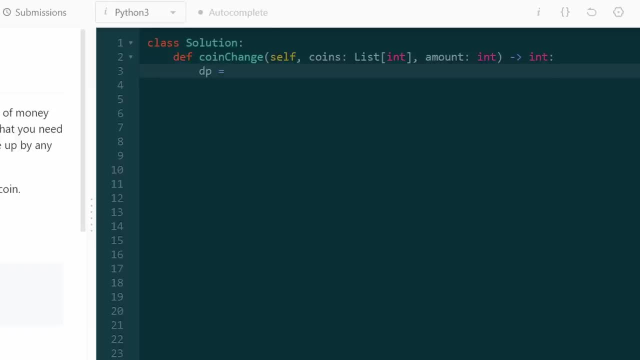 right. So from these four values that we computed, we want to take the minimum, which we know is two, So we can return two in this case. So that took us forever, But luckily the code is a lot shorter, Just like we showed. I'm going to have a DP array And I'm going to initialize this to be: 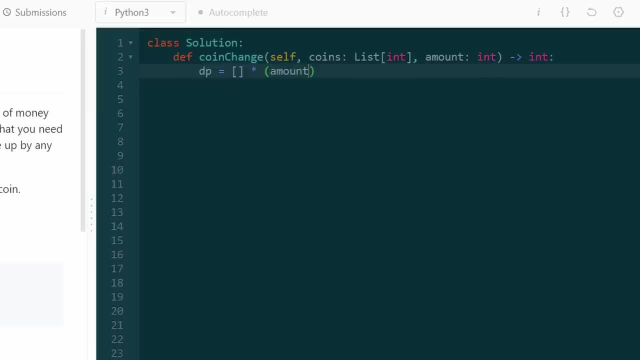 length of amount plus one, because we are going from zero all the way to amount And the default value I'm going to give each element in this array is amount plus one, Or you can do like infinity or whatever. the max int is like math dot max. 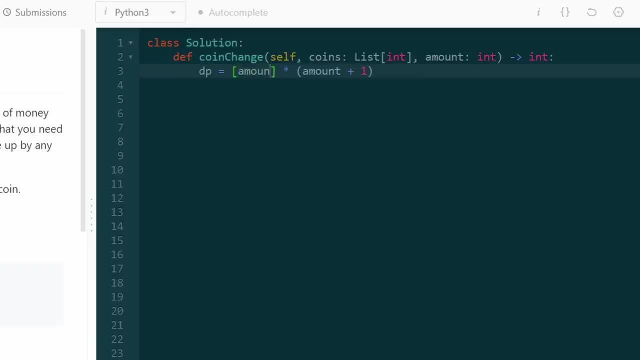 But amount plus one is basically a max value anyway, And we know that the base case for this is the DP of zero, meaning if we want to compute amount zero, that it only takes zero coins. And now we're going to start computing every value in DP, So for every amount A in range. 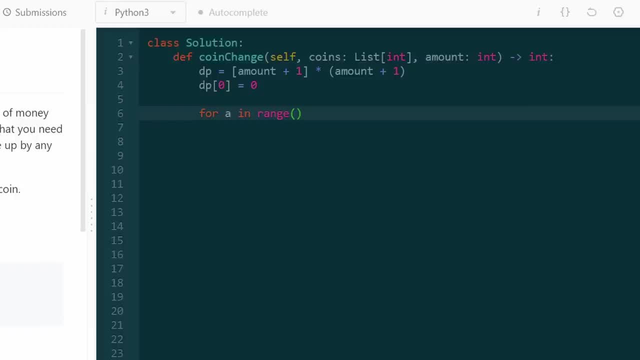 and we're going to do this in reverse order, not, or rather bottom up. So we're going to go from one all the way to the amount, And we, technically, are still doing it in a brute force way. So we are going to go through every coin, So for coin, in our list of. 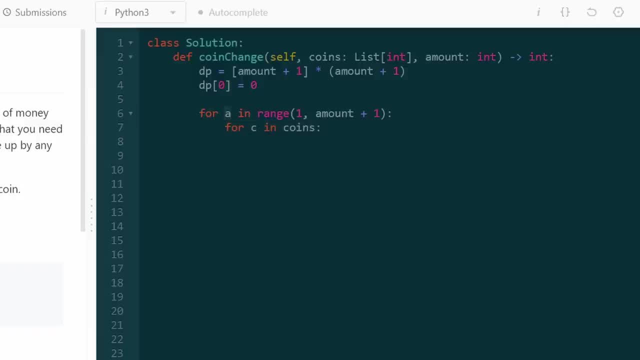 coins. So we're trying to compute this A amount. So we're going to take A and subtract the current coin that we're looking at. if this is non-negative, So if it's greater than or equal to zero, that means we can kind of compute the amount. So we're going to take A and subtract the current. 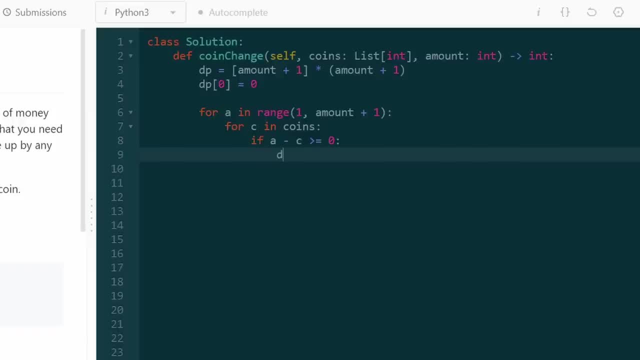 coin that we're looking at And we continue searching, right. So this means we possibly found a solution for our DP. So for this amount A, we're going to set it to the minimum of itself and one plus DP of A minus C. So this one comes from this current coin that we're using, C. 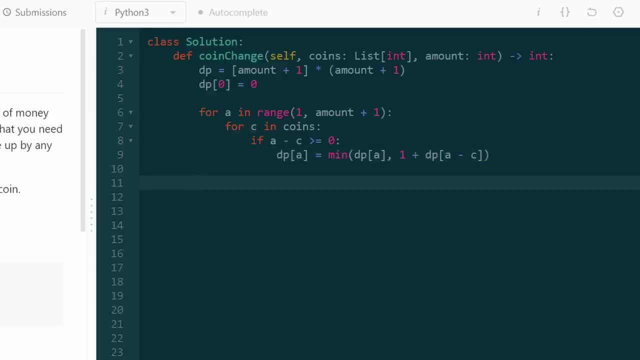 and DP of A minus C comes from. for example, let's say our coin is going to be A minus C, So this one comes from this current coin that we're using. C value was four and our amount that we're trying to compute A is seven. Basically we're saying DP. 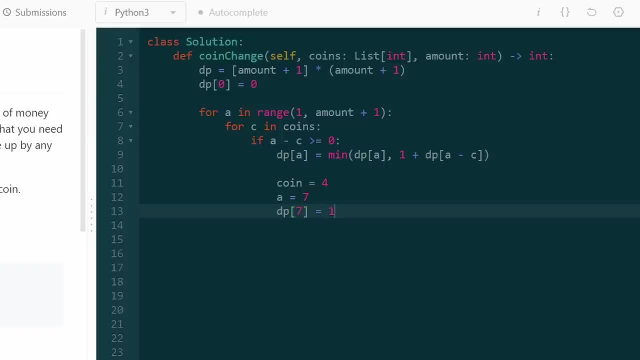 of seven is equal to one plus DP of three, because seven minus four is three. So we're saying that this is a possible solution, And actually that's the only thing that we have to do. This is basically it. This is like what's called the recurrence relation, And so now the only thing we have to do is return.